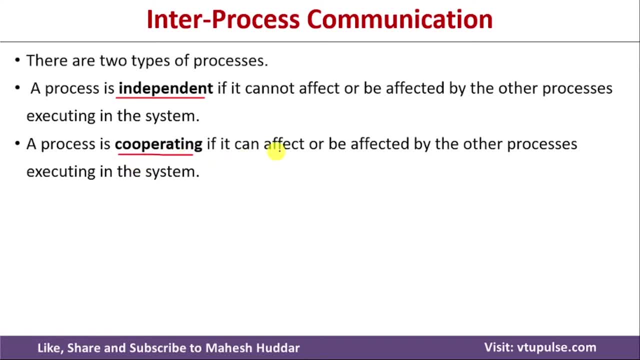 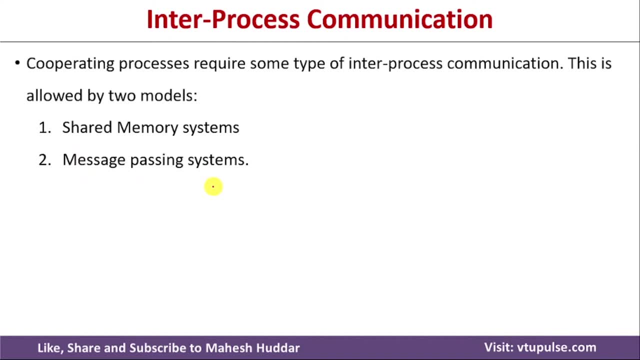 process. A process is cooperating if it can affect or gets affected by other processes executing in the system. over here, Whenever we have a cooperating processes in a system, we need to establish some inter-process communication strategy so that they can share the information over here. 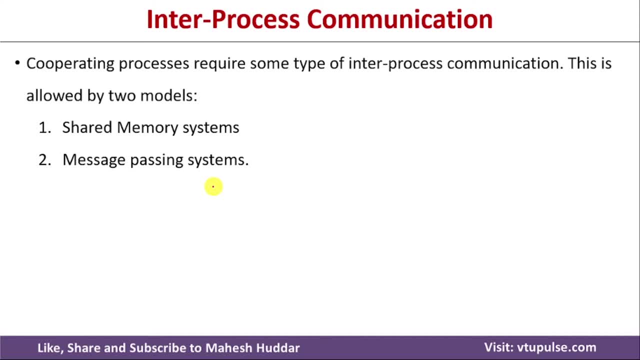 There are mainly two kinds of inter-process communication exist in operating system. One is known as shared memory system, Another one is known as message passing system. We will try to understand each of these particular methods in detail, one by one. The first one is known as: 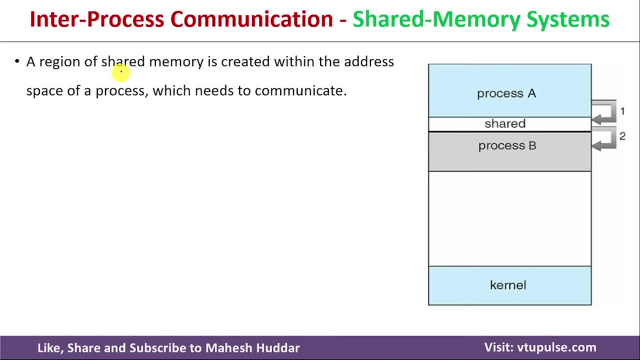 shared memory system. In this case, a region of shared memory is created within the address space of the process which needs to communicate. For example, in this case, let us say that process A and process B want to share some information. So first we need to create what? 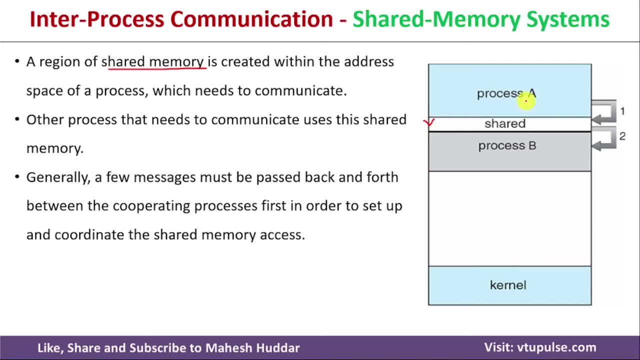 is called as the shared memory here. Whenever A wants to send some information, that will be placed into this particular shared region. Whenever the information is available on shared region that will be read by this particular B so that A and B can communicate with one another in this. 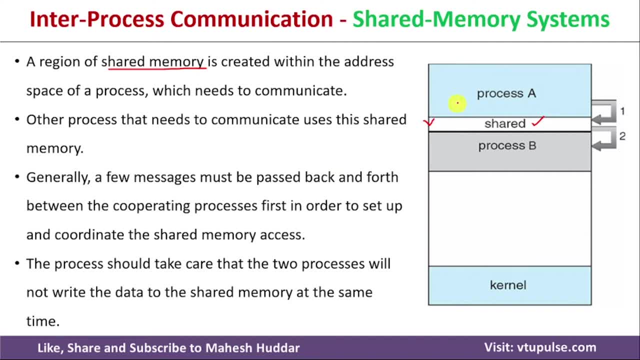 particular case here. So this is a simple strategy, what we can follow- that is known as shared memory system over here. But one very important thing we need to remember when it comes to shared memory: whenever we don't have a space into this particular shade memory, the process a has to wait because 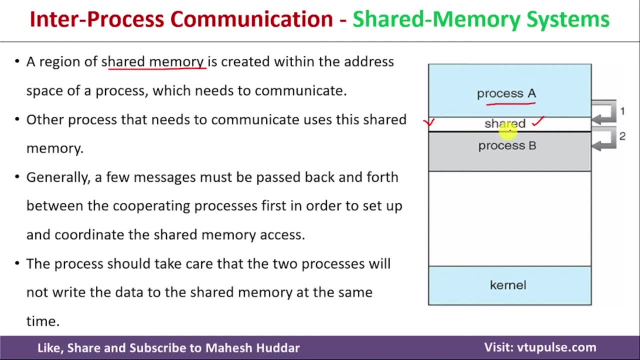 there is no space onto this particular shade memory and if you don't have any message on this particular shade memory, the process b cannot read that particular thing. so at a particular point of time, either process a can use this particular shade memory or process b can use this particular. 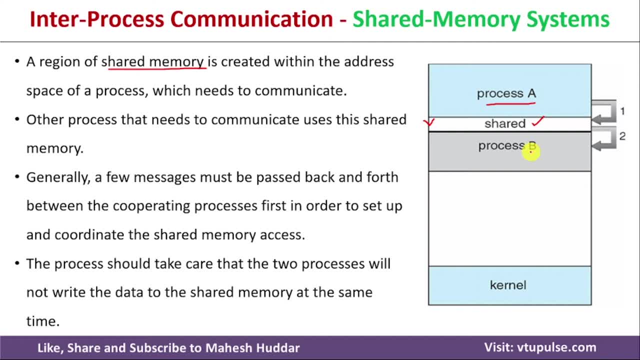 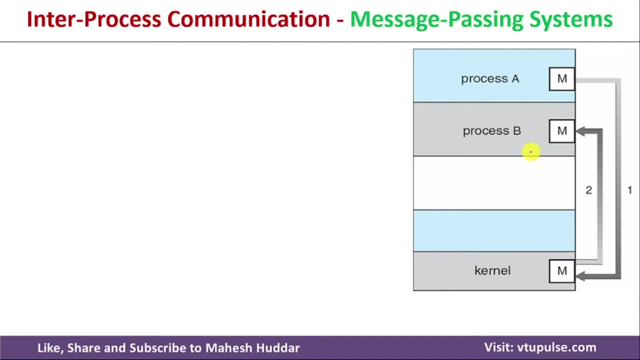 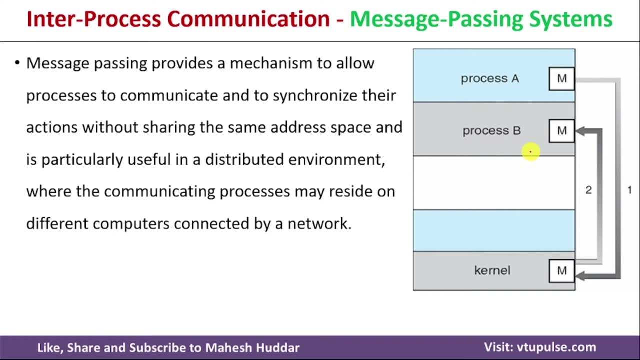 shade memory, not a and b at the same time over here. coming back to the second type of inter process communication that is known as message passing system, again, in this case, process a and b wants to communicate with one another. so what they do over here is they will send that particular. 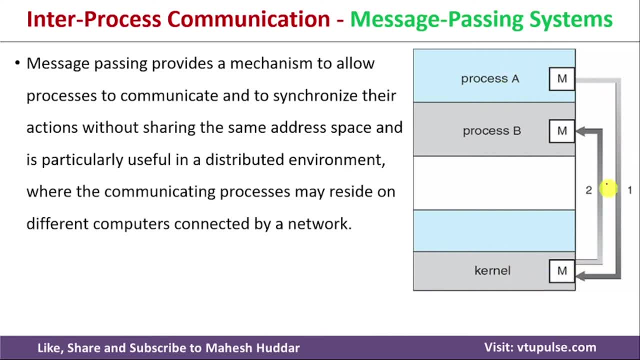 information to this particular kernel. from that particular kernel again, the particular message will be delivered to the destination over here. so this is how actually the inter process communication takes place in message passing system, and whenever you want to implement a message passing system in operating system, you can do that by using the inter process communication that is known as message passing. 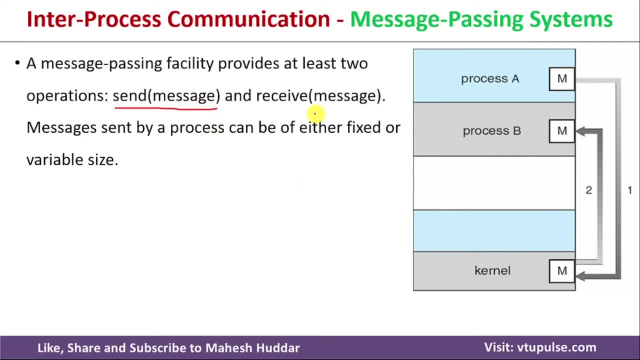 system we need to have at least two operations. one is known as send message and second one is known as receive message. over here, the size of this particular message may be fixed or variable. there is no question in this particular case if process p and q wants to communicate with another. 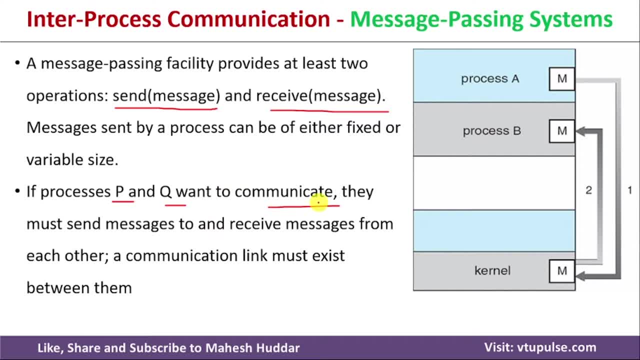 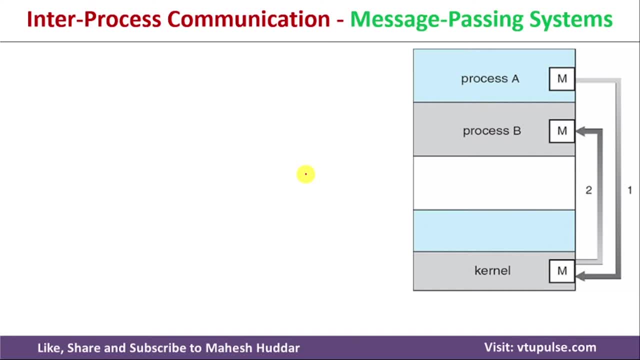 either of those particular processes should send a message and another one should receive the messages over here or the communication link between those two processes here. now there are some different types of message passing system exists in operating system. one is known as direct or indirect communication. second one is known as synchronous or asynchronous communication and the third one is known as 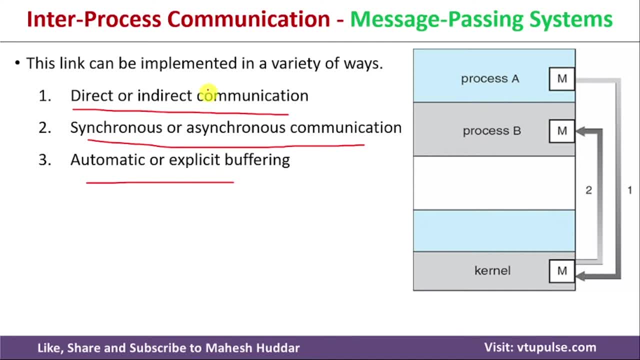 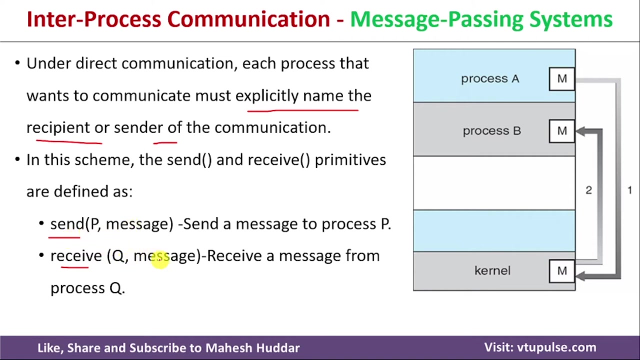 automatic or explicit buffering in this particular case. now we will try to understand each of these body things one by one. the first one is direct communication. in direct communication, each process that wants to communicate must explicitly name the recipient or the sender. over here, for example, the send and receive will look something like this here: send p comma. message, receive q comma. 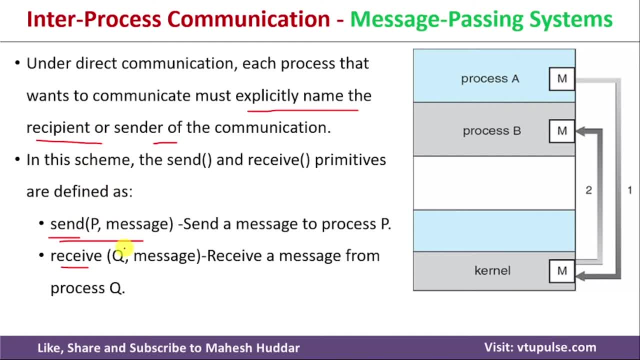 message here. what is the meaning of this one? the meaning of this one is a particular process which has executed this particular statement is trying to send a message to process p here. that is what the meaning of this particular statement. so what is the meaning of this one? the process which has. 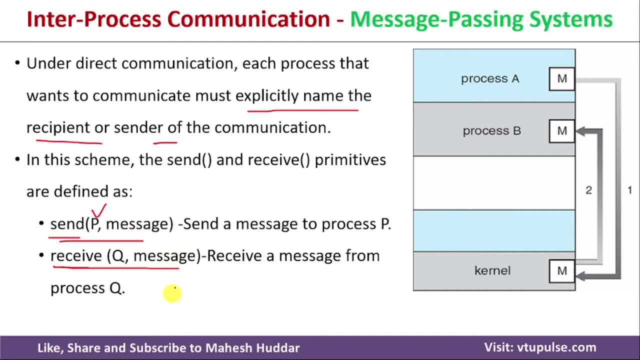 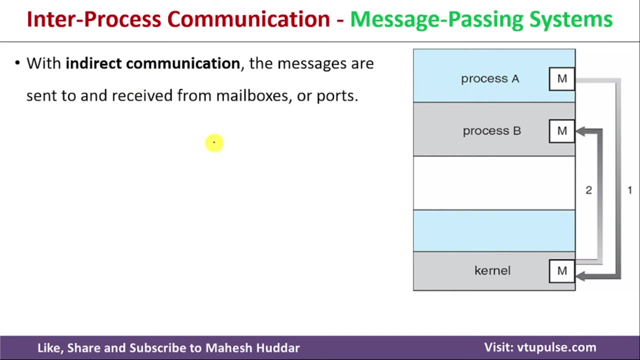 executed this particular statement that is received, q comma message. the meaning of this one is: the process is waiting for some message from q here. so that is what the meaning of send and receive in this particular case. in indirect communication, the messages are sent and received using something. 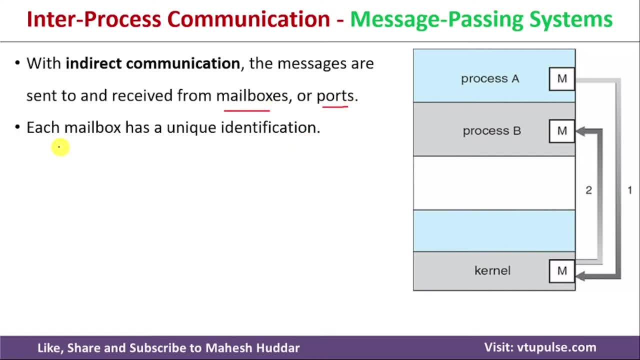 called as mailboxes or the ports over here. so each mailbox has a unique identification number. in posix we use integer numbers to identify those particular mailboxes. over here the two processes can communicate only if the processes have the shared mailbox. for example, we have created one mailbox here. a and b can communicate with one another or can say that. 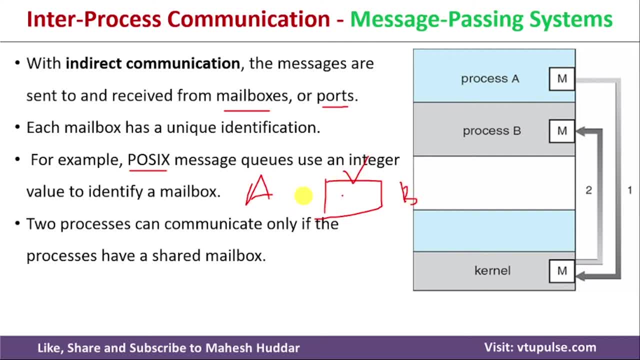 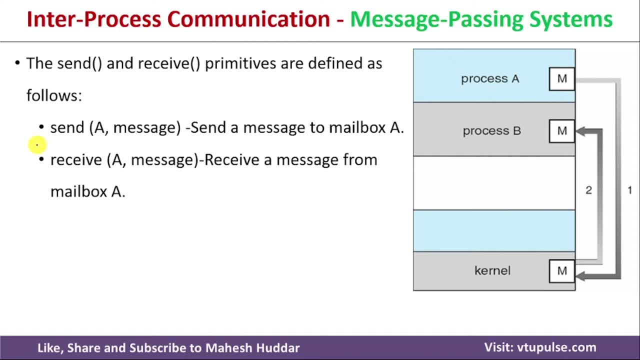 the two processes, a and b, can communicate with one another if they have the shared mailbox in this particular case. so now how send and receive will look like in indirect communication is. the send will look something like this: send a comma message. the meaning of this one is: 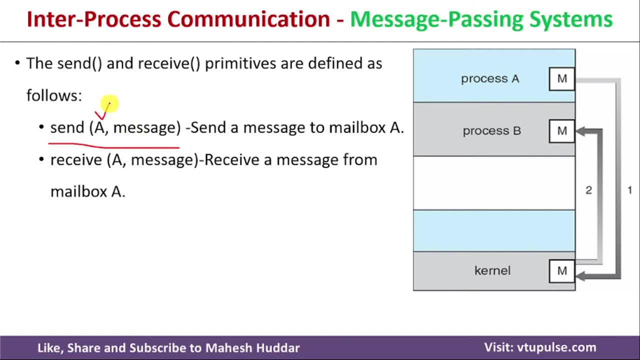 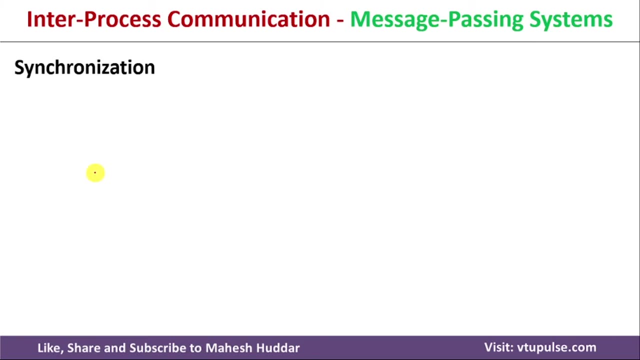 send a particular message to this particular mailbox a here and receive a comma message means the process is going to receive a message from this particular mailbox, a in this particular case. now coming back to the next one, there is something called as synchronization, or you can say that: 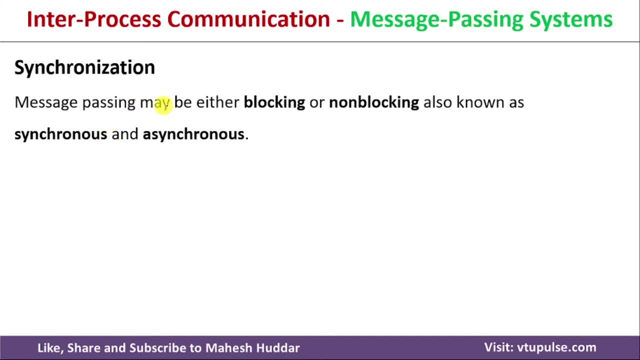 synchronous or asynchronous message passing. the synchronous and asynchronous message passing is also known as blocking or non-blocking message, passing over here. now, what is blocking? there are two kind of things can exist: blocking send and blocking the receive over here. in. blocking send whenever a particular process is sent to a particular mailbox, a in this particular case. 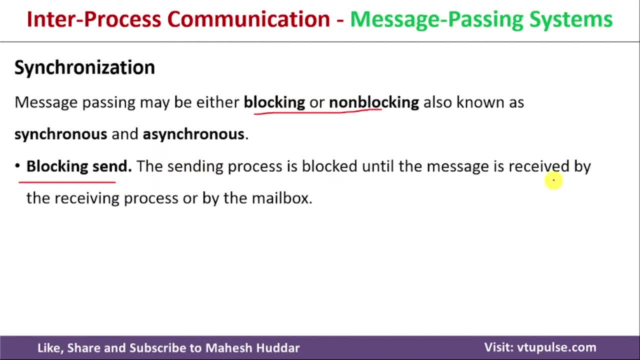 it will not block its send here and there will be block whenever specific process has sent a message. it will block itself until that particular message is received by the receiver, in this case, or that particular message has been put into this particular mailbox. so that is what called as blocking send. in this case, what is non-blocking send, and whenever. 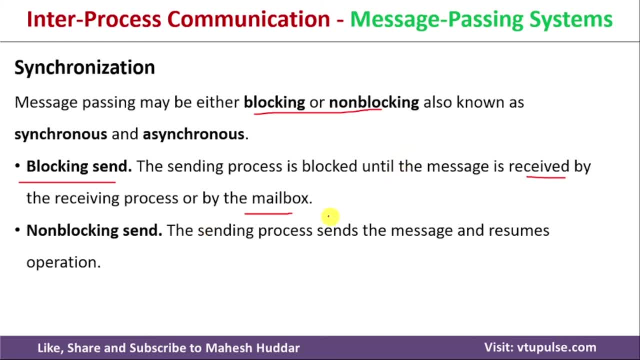 a particular process sends some message to another process, it will not block itself or it will not wait for that particular message to be delivered. it will continue it's work without waiting here. so that is what is called as non-blocking send in this particular case. coming back to the third one, only that the individuals have sent a comma message here. 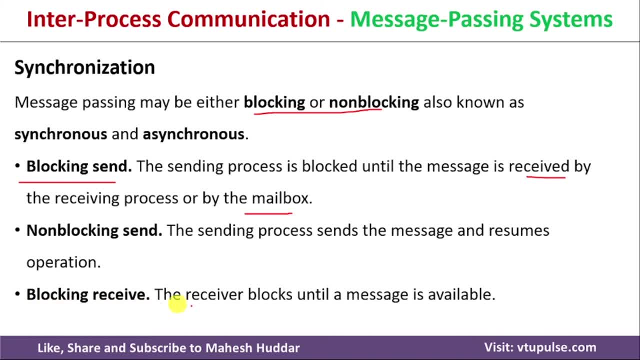 that is a non-blocking process. so in this case we have says: heard everything. the write one that is known as blocking receive. the receiver is waiting for some message, and if that particular message is not available in mailbox, then it has to wait here. so that is what is called as a blocking. 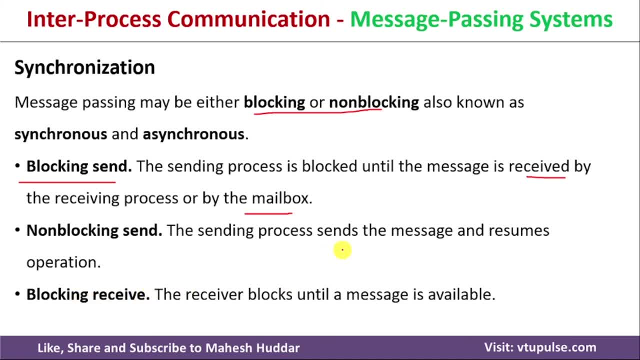 receive. in this particular case, it is not doing any other work it is waiting for. we can say that the message to be received over here, the last one, is something called as non-blocking receive. a particular process has made a request for a message. if it is available, it will be delivered. 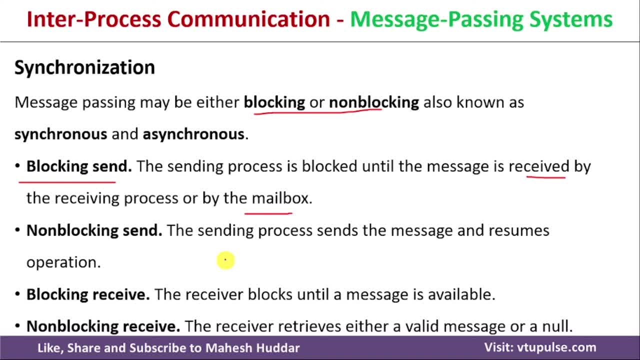 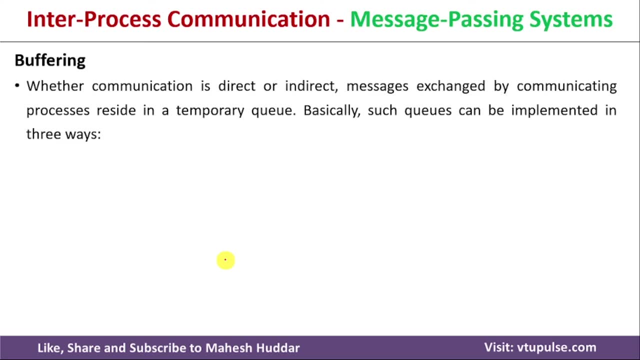 well in advance: if it is not available, that particular process will not be blocked over here, that the remaining process, or you can say remaining tasks, will be continued by that particular process over here. the last part of our discussion is something known as buffering in message passing system. so whenever we establish a communication channel from, you can say that. 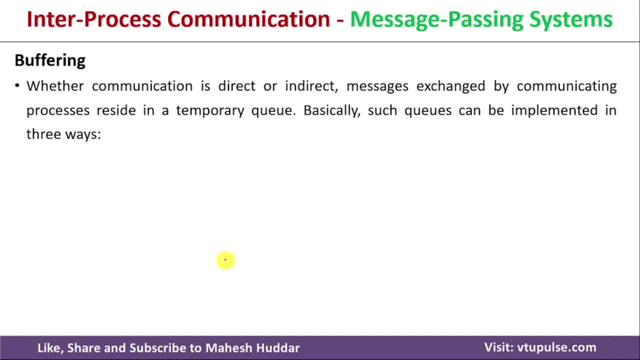 one process to other process, either in direct or indirect mode. what actually happens over here is, uh, the. the message which has been sent by the sender has to be stored into something called as a temporary queue. once that particular message is available in temporary queue, the receiver can receive that particular message here. basically, that particular